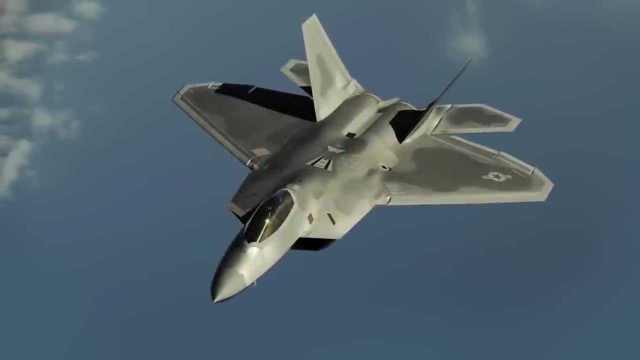 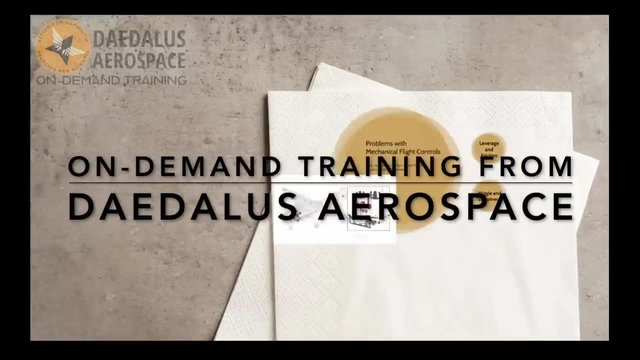 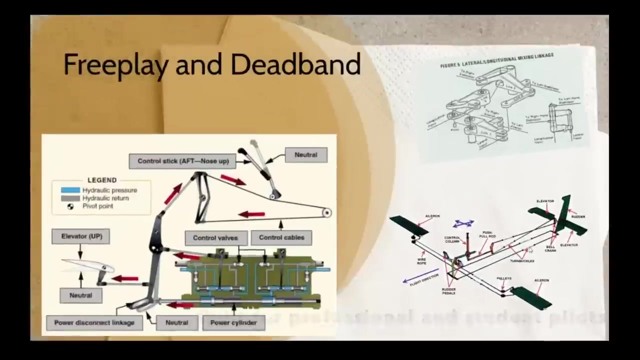 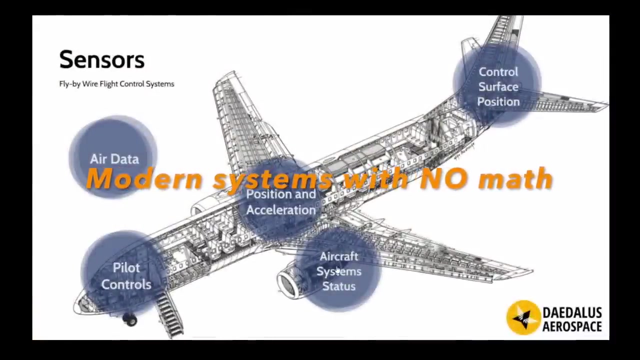 Please subscribe to the channel and press the bell icon to receive notifications when I upload a new video. Thank you for watching. See you in the next video. 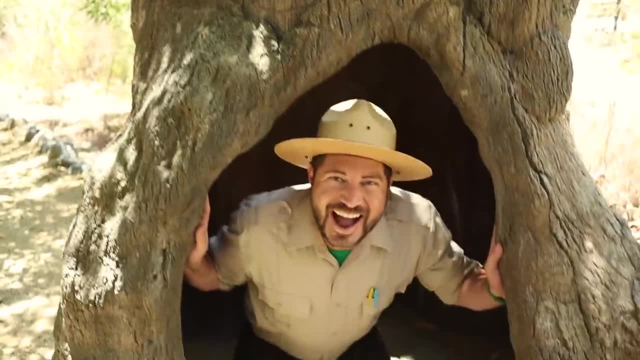 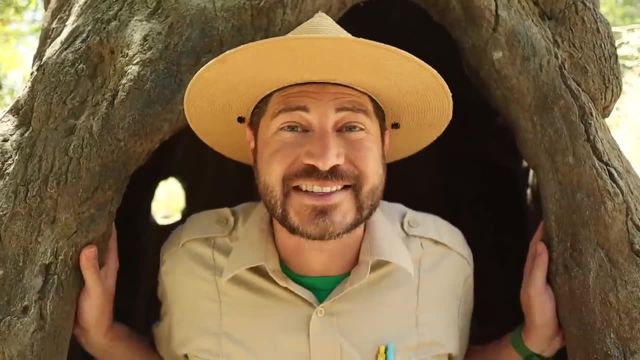 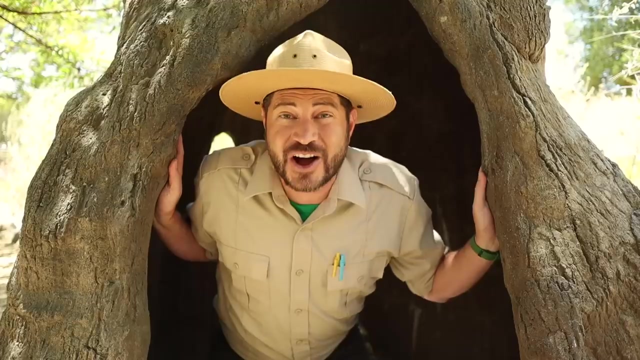 Howdy Junior Rangers. Welcome back to the Ranger Zach Show. I want you to think about your home. What makes it a safe place for you to live? Do you got it Well? did you know that all plants and animals on earth need safe homes, just like you And the special places that plants and animals 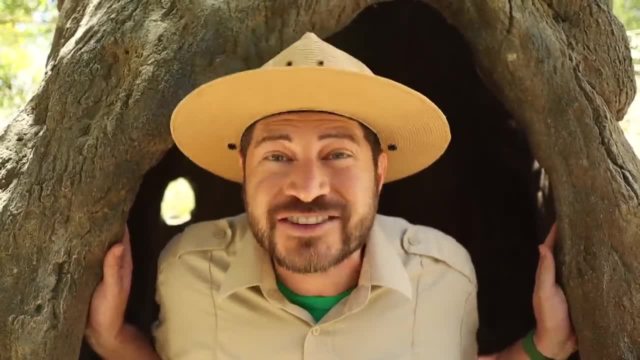 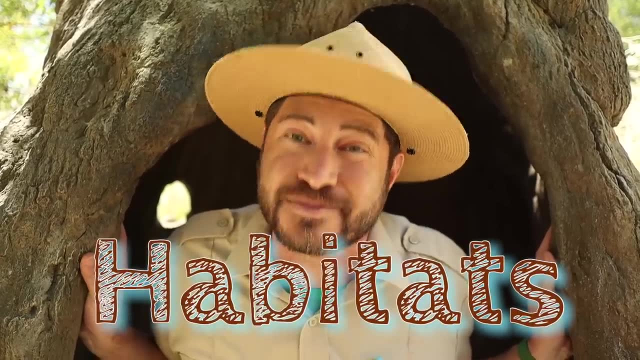 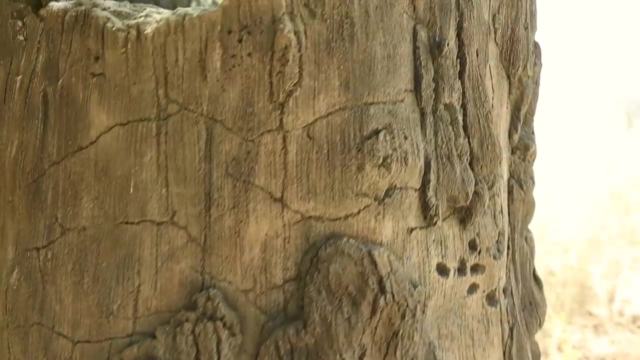 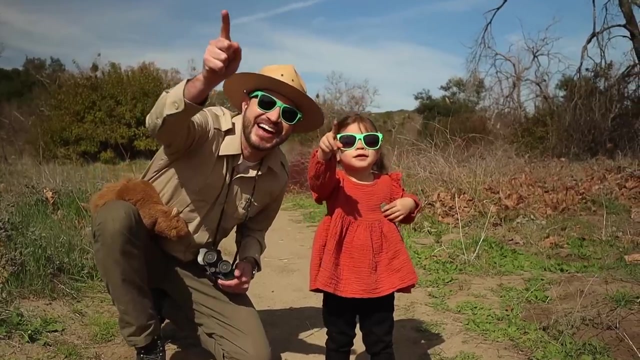 make their home is called habitat, And that's what we're going to learn about today. So pack your bags and come along for another very exciting adventure as we learn how habitats make a home. If you ever want to know what makes a tree grow tall, a white turtle wears a shell on its back. 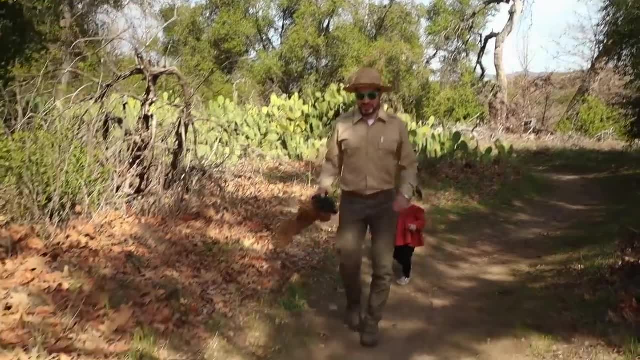 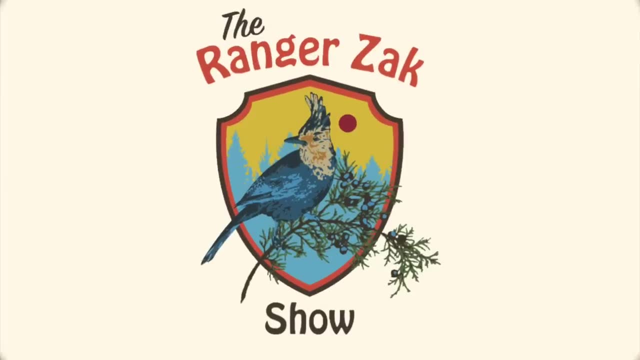 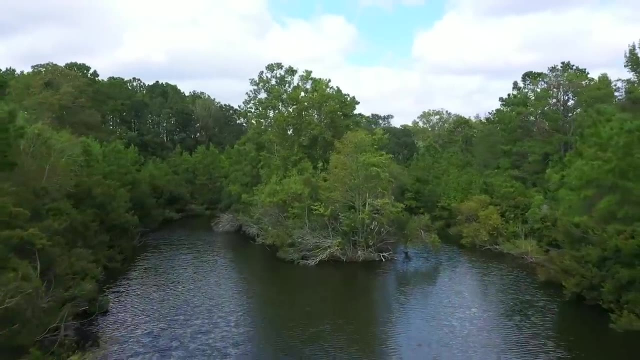 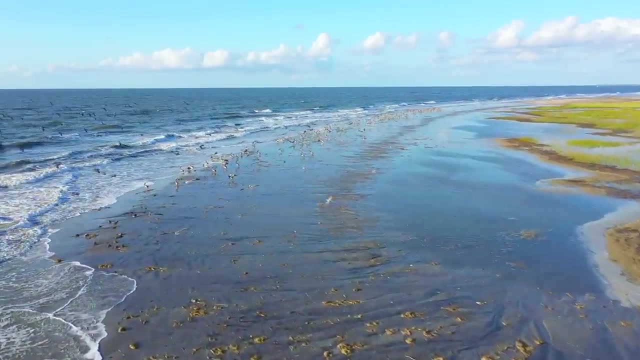 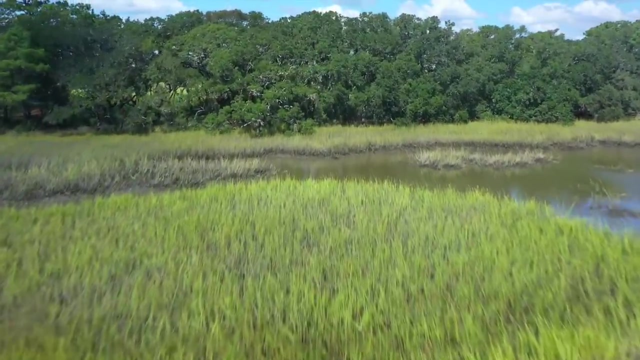 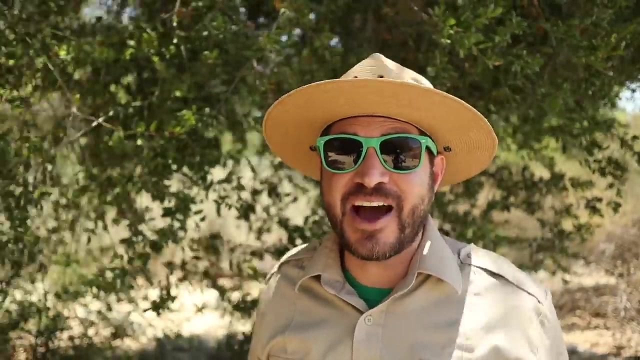 To get your hiking boots and a walking stick. come along with Ranger Zach. Come along with Ranger Zach. It's the Ranger Zach Show. So there are many different types of habitats that can be found throughout the world, like mountains, forests, deserts and grasslands, And obviously, 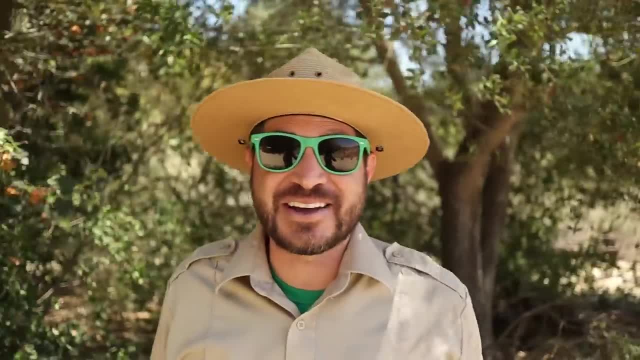 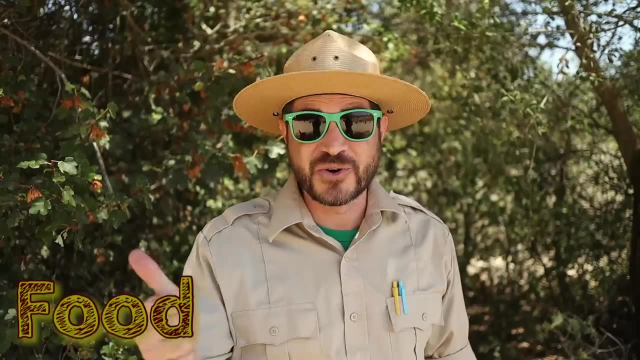 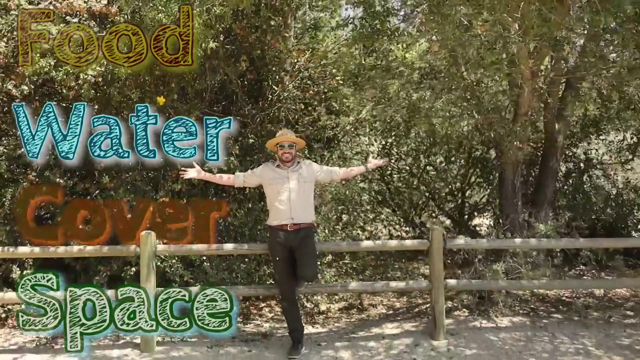 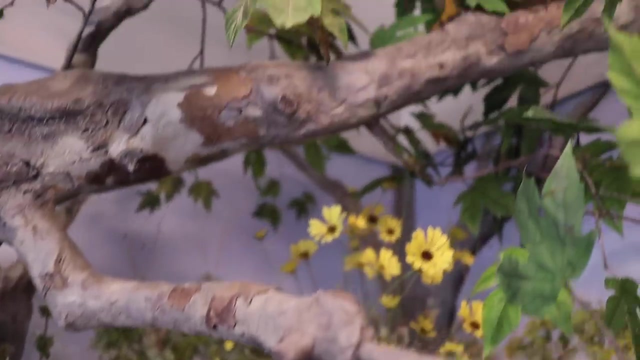 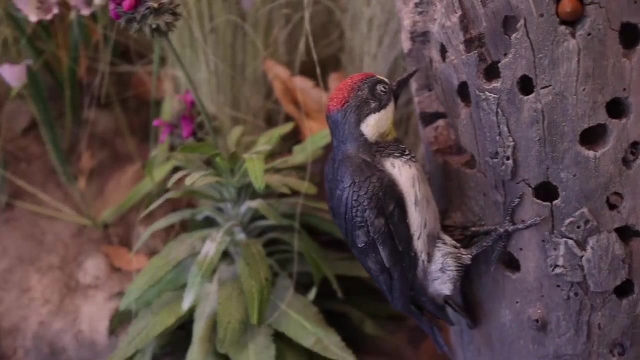 each one is special and different. So what makes a habitat well a habitat? Well, for a habitat to make a good home, it needs four special ingredients: Food, water, cover and space. Now, what do you think about the three most significant habitats that can be found in the world?